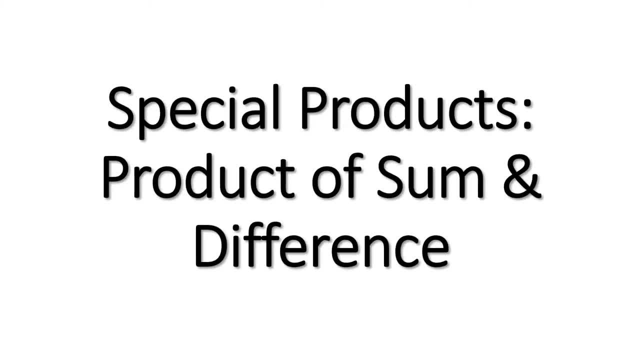 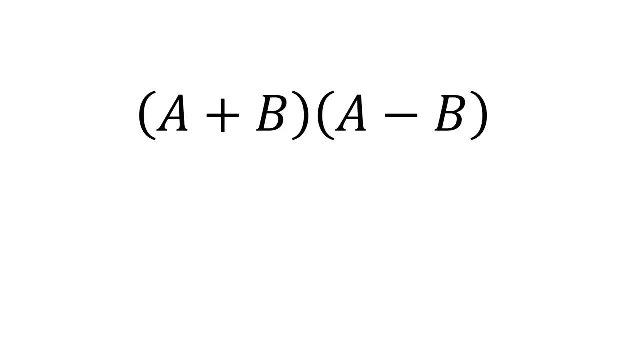 In this video we're going to learn a shortcut in multiplying a special product, the product of sum and difference. Let's say we have a plus b times a minus b. Now, using the FOIL method, this is equal to a squared minus ab plus ab minus b, squared Negative ab plus ab is zero. 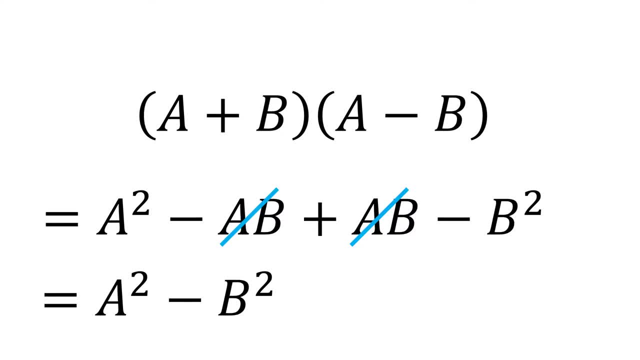 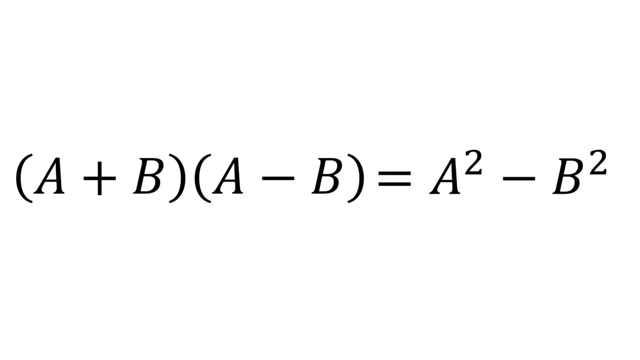 So this is equal to a squared minus b squared. So therefore, a plus b times a minus b is equal to a squared minus b squared. Now, using this formula, we can quickly find the product of the sum and difference of two terms without using the FOIL method or the distributive property in. 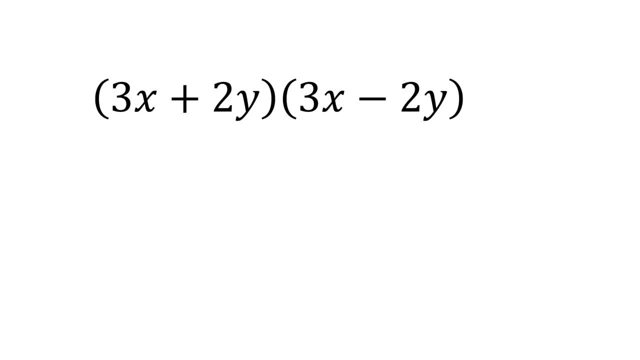 general. For example, let's say we have three terms. Let's say we have three terms. Let's say we have three x plus 2y times 3x minus 2y. In this case we have a as 3x and b as 2y. 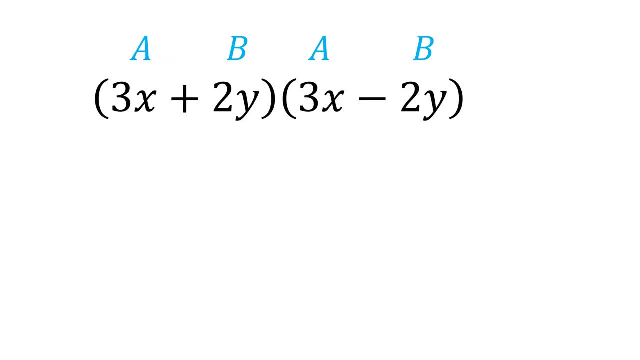 Now, instead of using the FOIL method, just take the square of 3x, then subtract the square of 2y, which is equal to 9x squared minus 4y squared. So therefore 3x plus 2y times. 3x minus 2y is equal to 3x plus 2y. Now let's take the square of 2y, then subtract the square of 2y, which is equal to 9x squared minus 4y squared. So therefore 3x plus 2y times 3x plus 2y. 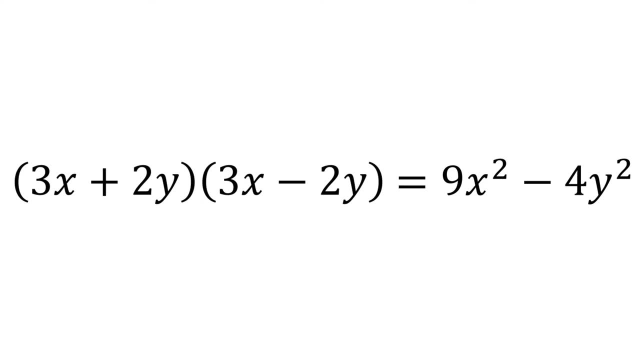 3x minus 2y is equal to 9x squared minus 4y squared. Now let's say we have 2x plus 5 times 2x minus 5.. In this case, we have a as 2x and b as 5.. Now, instead of using the formula method, 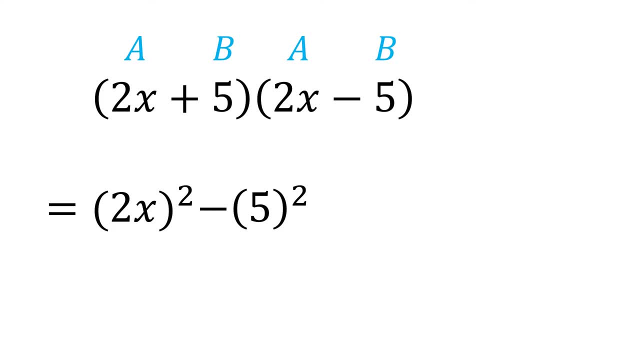 just take the square of 2x, then subtract the square of 5, which is equal to 4x squared minus 25.. So therefore, 2x plus 5 times 2x minus 5 is equal to 4x squared minus 25.. If we have,